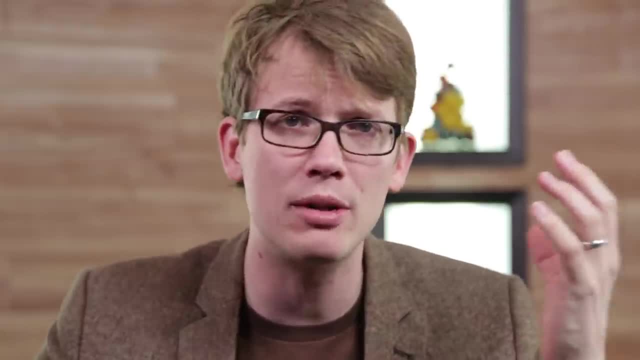 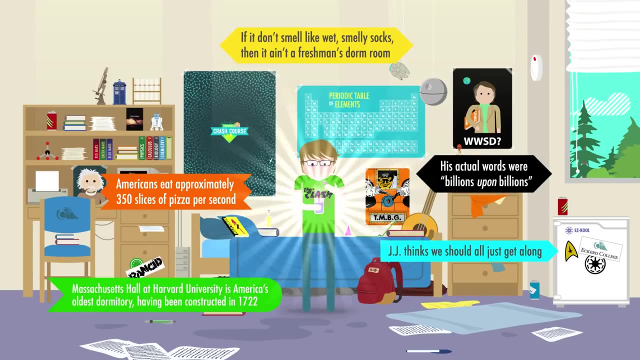 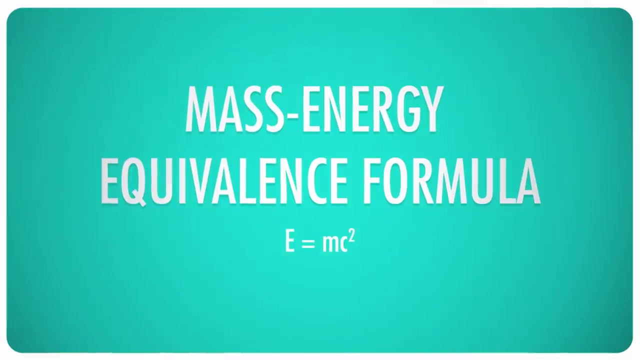 But it's probably also famous because it's important. It explains one of the most powerful sources of energy known to humanity. E equals mc. squared is formerly known as the mass-energy equivalence formula, and it states that mass is interchangeable with energy. Okay, there's a lot there in what I just said. 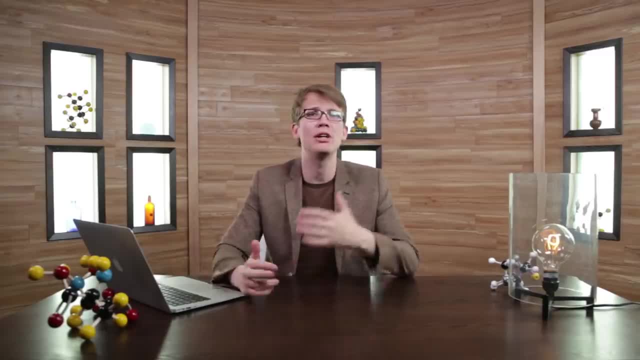 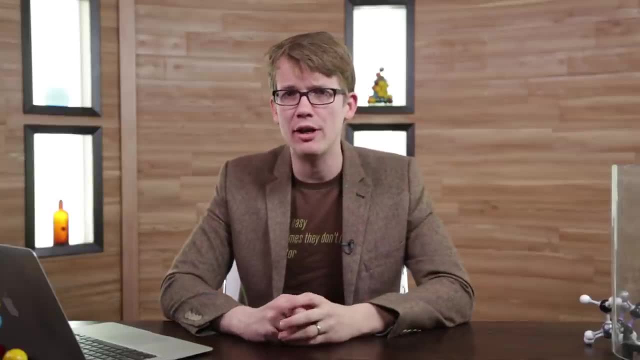 To tease it apart, consider the nucleus of an atom of oxygen: eight protons and eight neutrons Collectively. by the way, these particles are known as nucleons. If you were to add up all the individual masses of all 16 nucleons separately and then compare that to the total mass of an actual oxygen nucleus, 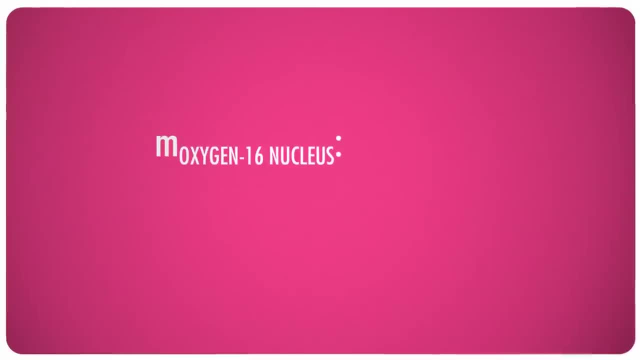 you'd find that there's a difference between the two. This nucleus, exactly 15.99 atomic mass units, is lower than the mass of its individual nucleons put together, In this case 16.13 amus. That mass went somewhere. 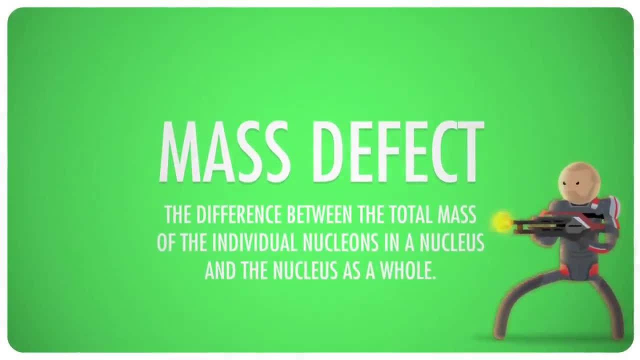 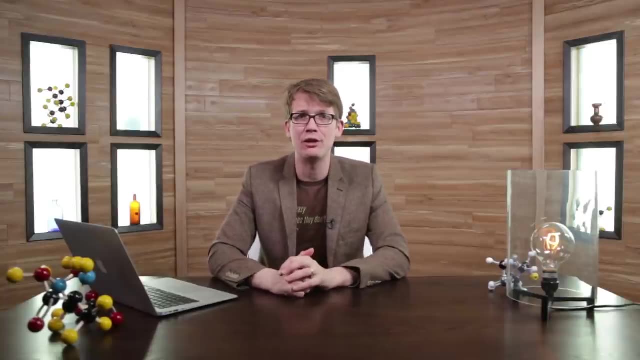 That missing mass in the nucleus, known as its mass defect, is actually present in the form of energy. It's the energy that holds the nucleons together. So, for example, the mass defect for an oxygen atom is negative 2.269 times 10 to the negative 28th kilograms. 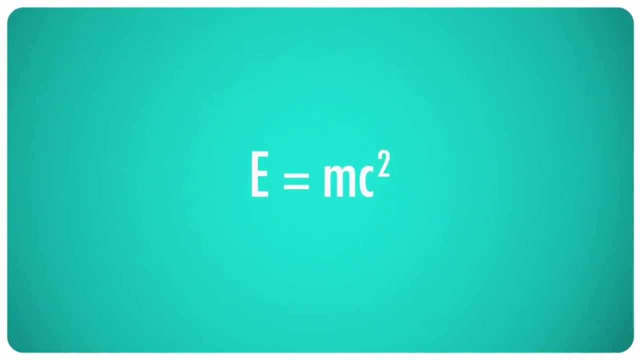 To find out how much binding energy that missing mass amounts to, you can use it as the mass of an atom. That's the M in Einstein's formula. This ingenious little equation relates mass and energy by a simple proportionality constant and thanks to Einstein we know that constant is the square of the speed of light, or C squared. 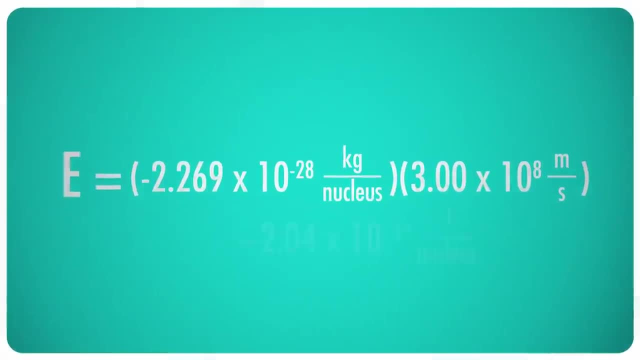 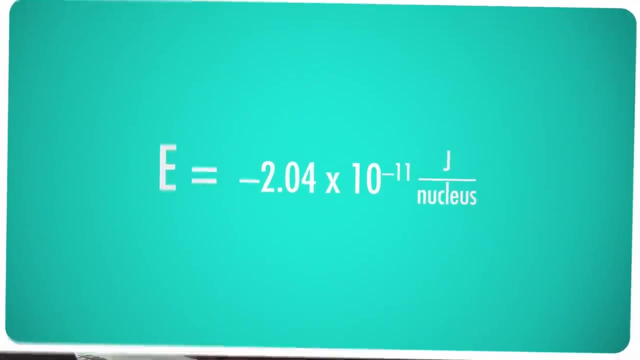 Solve for E and you find that the binding energy in that oxygen nucleus is 2.04 times 10 to the negative 11th joules, with the negative sign indicating that the energy is being released. Now, of course, 2.04 times 10 to the negative 11th is a very small number. 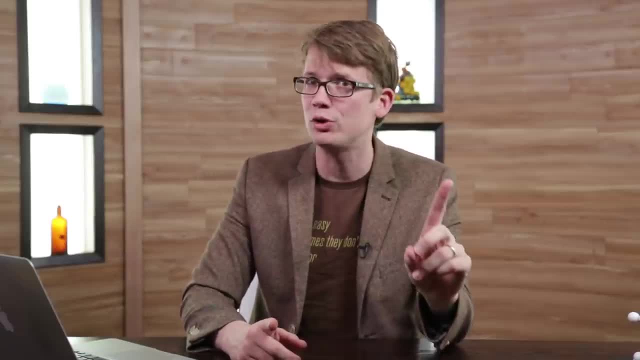 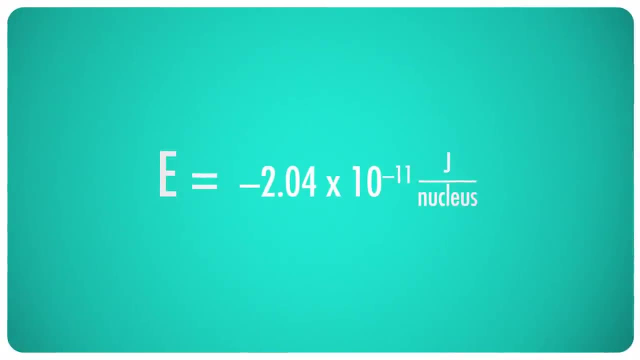 That might surprise you, but hold the phone. That is just for one single nucleus. If we multiply that by Avogadro's number to find the energy change for a whole mole of oxygen nuclei, a mere 16 grams of oxygen, we get an amazing 1.23 times 10 to the 13th joules of energy. 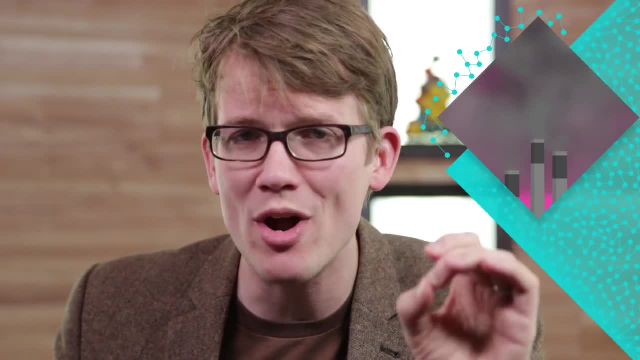 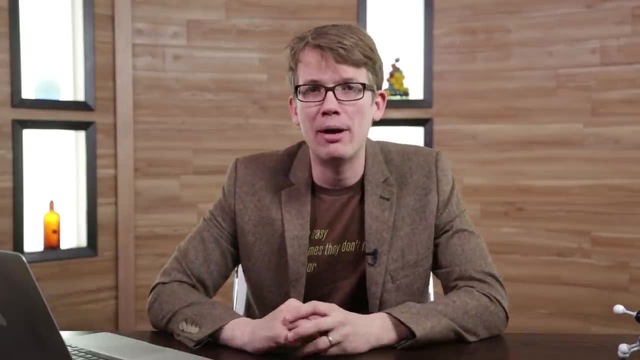 To produce that energy with coal, you would have to burn 420,000 kilograms, 420 metric tons of coal. That energy is what we mean when we talk about nuclear energy: the binding energy that's released when a nucleon is removed from its nucleus. 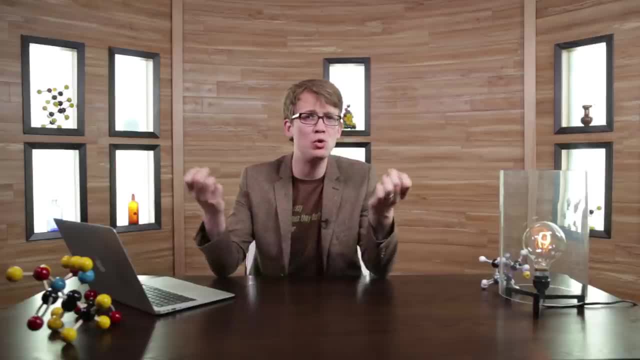 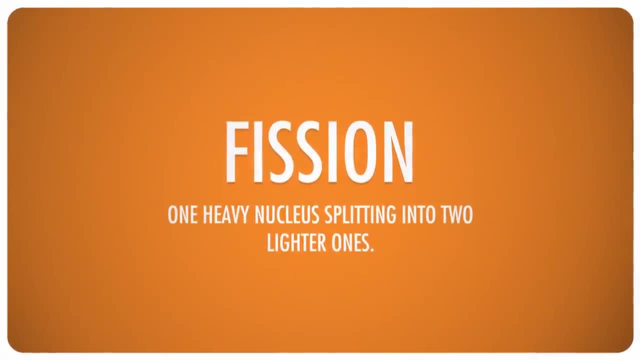 To dislodge one of those nucleons and unleash that energy. there are two general types of nuclear reactions: fission and fusion. Fission occurs when a large nucleus splits into two lighter ones. Fusion is the opposite, when two light nuclei join together to form a heavier one. 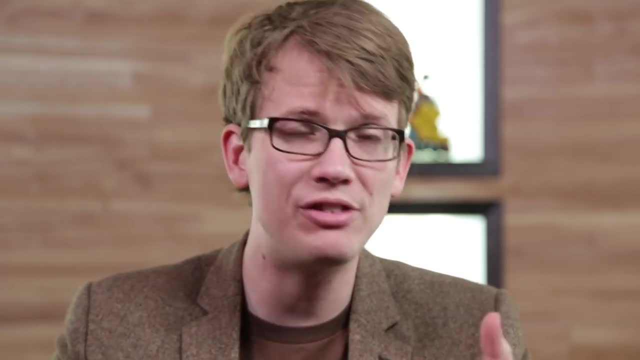 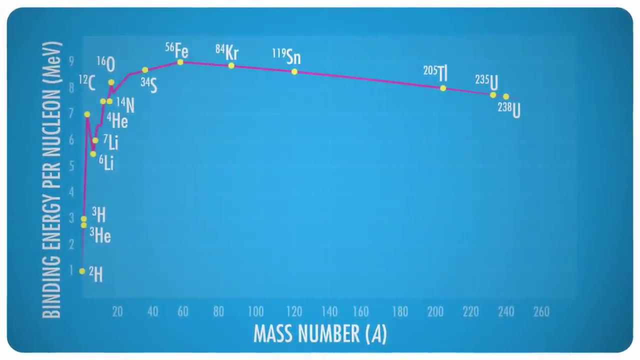 In both cases, the products of the reaction are more stable than the starting materials, and this is, as always, what drives the reaction. This is a graph of the binding energies of various elements compared to their mass numbers. Elements with very high binding energies, such as iron-56,. 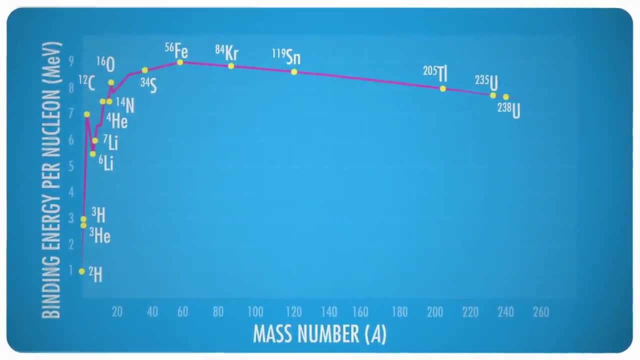 are very stable and rarely unstable. They can undergo nuclear reactions. but elements with lower binding energies can react much more readily. If the nucleus is heavier than iron-56, it will tend to break into two or more smaller nuclei- a fission reaction. 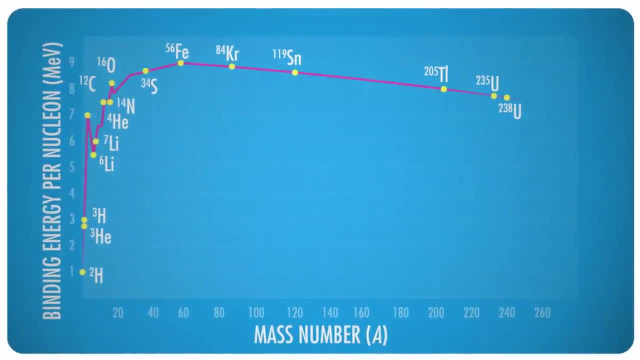 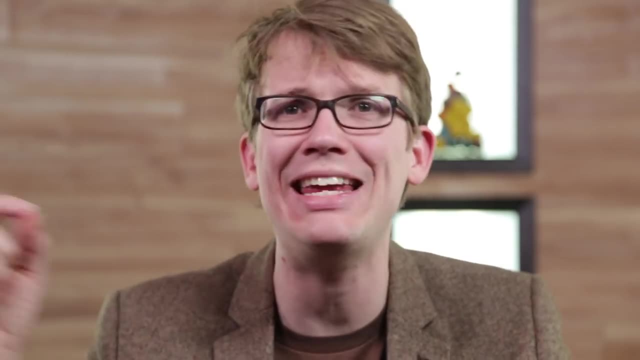 If it's lighter than iron-56, it will more likely participate in a fusion reaction, joining two nuclei together to form a heavier one. But the most important thing to notice here is that with both fission and fusion, stability increases as a result of the reaction. 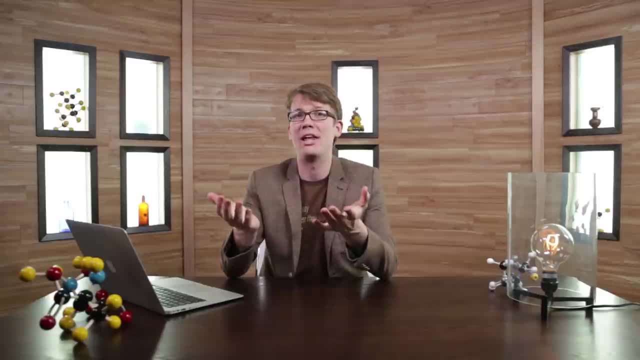 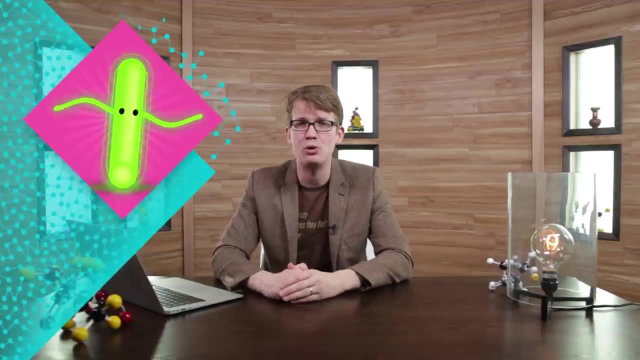 Fission is the type of reaction that we use more often because it's the one that we're better at initiating and controlling, at least so far, And whether it's used in power plants or bombs. the most common fuel for fission is uranium-235. There are several ways that it can react, but the reaction is almost always triggered by hitting uranium with neutrons from another source. When that happens, the uranium splits into smaller atoms. One such reaction produces krypton-92.. Yes, krypton is a real thing. 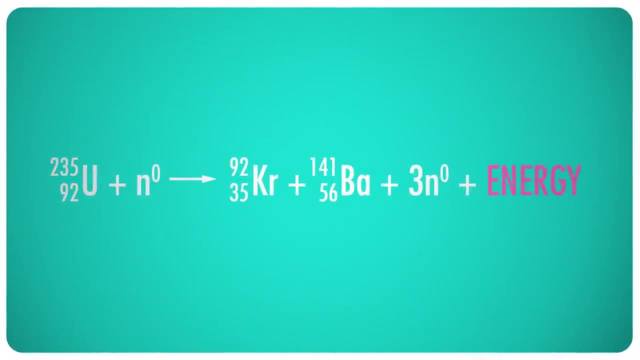 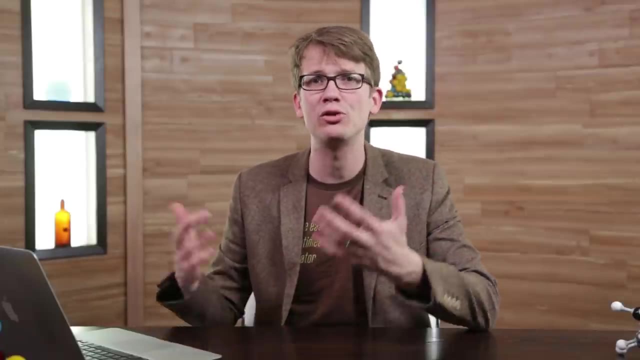 along with barium-141, three free neutrons and lots of energy. This energy is released mainly as the kinetic energy of the escaping particles, which is immediately transferred to the surrounding atmosphere. This energy is also released in the form of electromagnetic radiation. 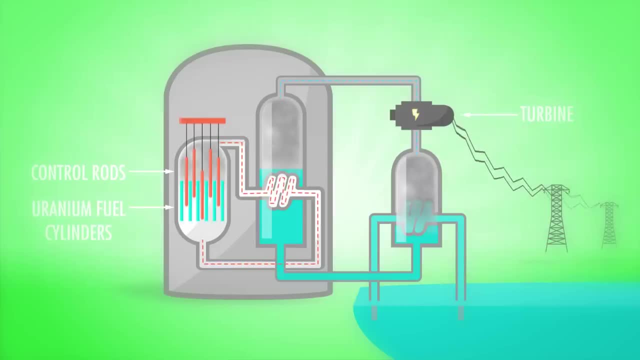 such as visible light, x-rays and gamma radiation. Nuclear power plants use the energy released by these reactions to convert water to steam, which then is passed through turbines spinning a generator, powering cities and stuff, Because of the enormous amounts of energy these reactions can release. 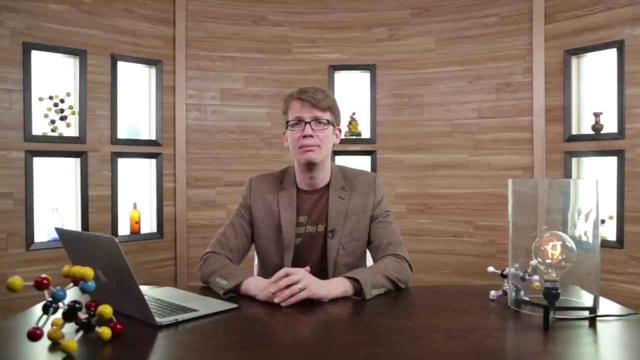 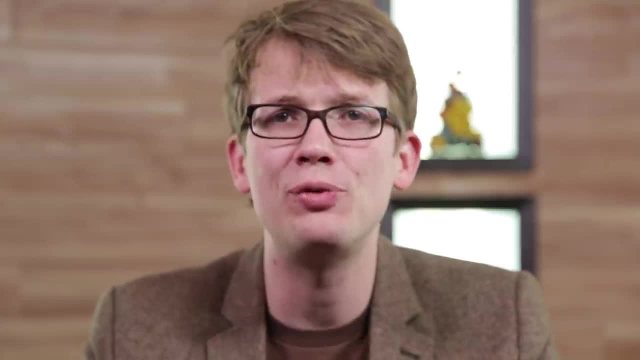 nuclear power plants can potentially produce lots of electricity. But there's also- I think you may have heard- some serious drawbacks. For one thing, as you know, atoms rarely exist in isolation. We write the equation of a fission reaction as if it's just one atom. 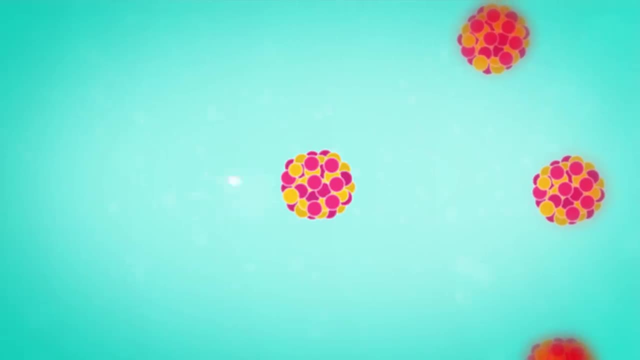 but in reality that one atom is surrounded by many, many more, And if one little neutron can trigger the reaction and that reaction liberates three more neutrons, well, I think you can see where this is going. If the reaction isn't controlled, each reaction triggers three more. 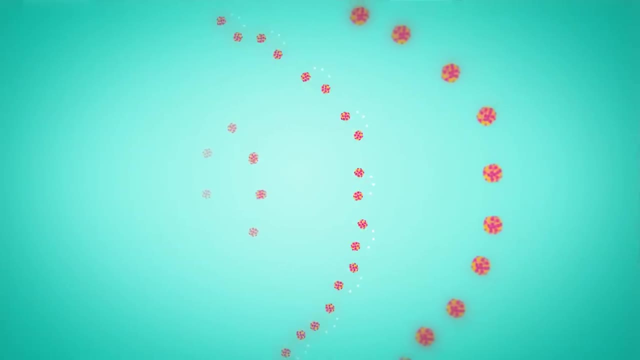 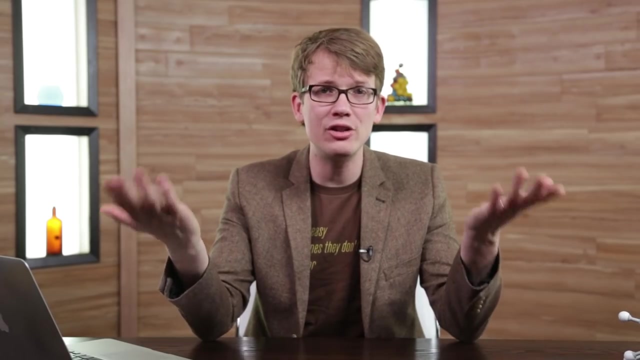 and every reaction releases the same amount of energy, which adds up fast. This is pretty much the definition of a chained reaction and it is the basis of the remarkable power of a nuclear weapon. The same type of reaction occurs in nuclear power plants. 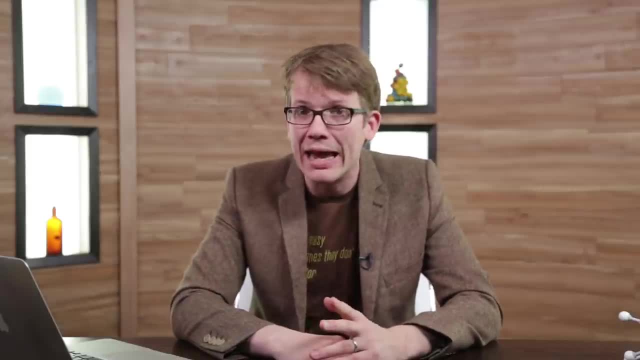 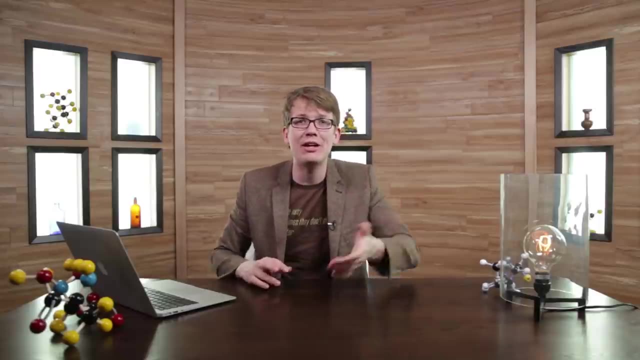 but those reactions are controlled in several ways to keep them from getting out of hand. The fact is, these chain reactions have the potential to produce far more heat than the plant can use, so much more that the temperature can easily rise to dangerous levels. 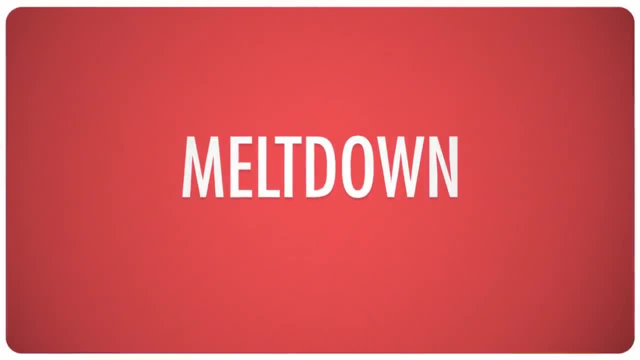 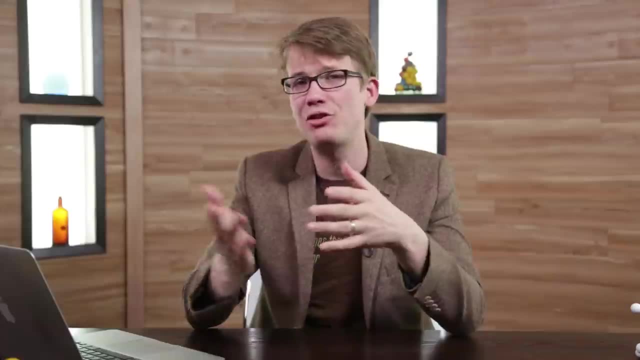 enough to melt the uranium- This is the meltdown that you hear about- and most reactor cores are immersed in water to disperse the heat and prevent this from happening. But that that's not enough on its own to control this thing If the chain reaction is allowed to run freely. 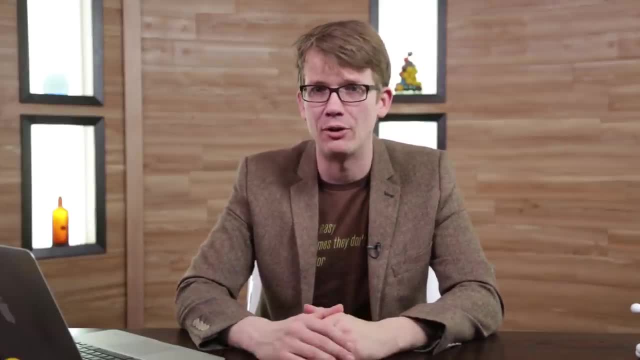 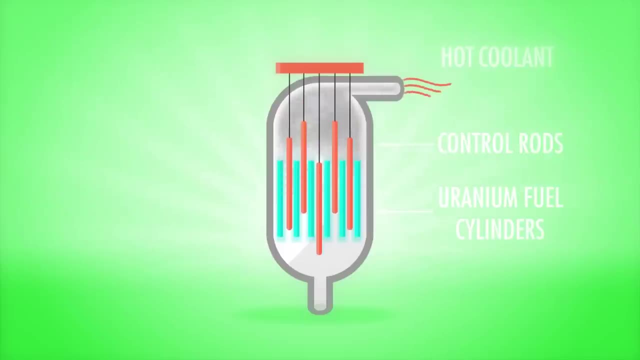 no amount of water can remove the heat fast enough to prevent a meltdown. The real way we control nuclear reactions is with control rods. They're made of materials that readily absorb neutrons and they're inserted between the fuel rods of uranium to slow the neutrons down. 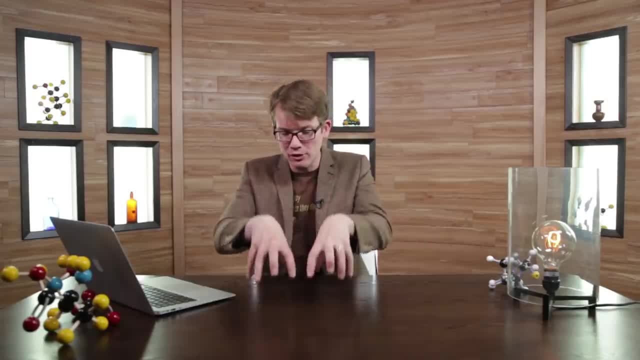 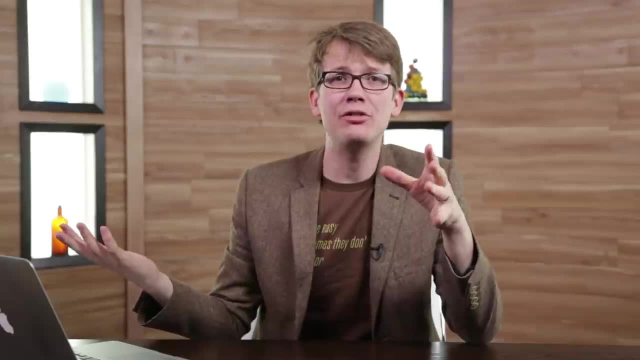 and therefore slow down the reaction. They can be put in more to slow the reaction more and lifted out more if you need more heat. Now, the other sticky wicket of fission reactions is the stuff that's left behind. These reactions not only produce products that are still radioactive, they produce tons of them, Lots of different troublesome kinds. Like we saw last week, uranium undergoes many different types of nuclear decay. so not only does each uranium atom produce isotopes of krypton and bromine, but that process also produces many other isotopes of other elements. And as these various nuclei break down, they release more neutrons and more unstable products, and the process continues for a long time. All of these reactions eventually yield stable products, but they have half-lives ranging from a few years to tens of millions of years. The products with shorter half-lives stabilize pretty quickly, but they release particles and energy like crazy during that time, so they're extra dangerous. The ones with longer half-lives decay more slowly, release less energy, but that means it takes a very, very long time. 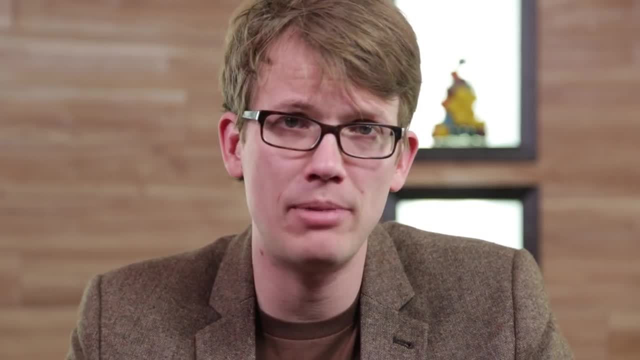 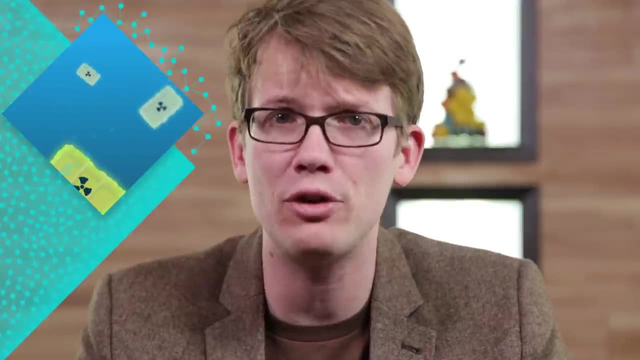 for them to stabilize So long, in fact, that for human purposes it may as well be forever. That means they'll always be an issue in our environment, which is why we're always looking for ways to store them and keep them out of our way. Fusion reactions, as you'd expect, are very different from fission. For one thing, the energy released in many fusion reactions dwarfs even the huge amount released by fission. You might be familiar, for example, with the wonderful work done by our Sun. 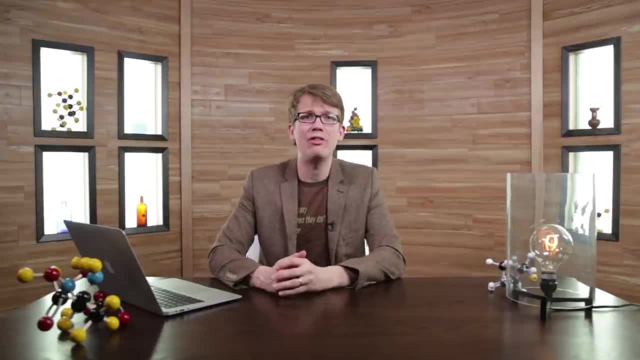 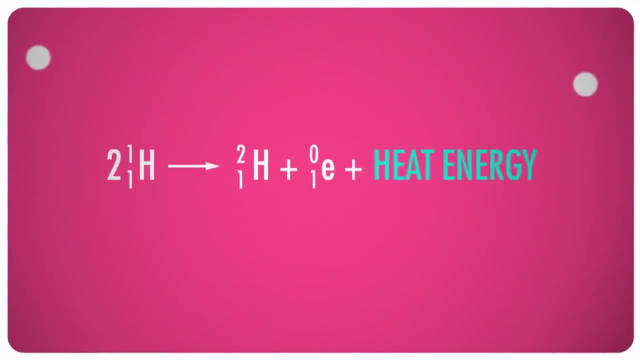 The reactions that power the Sun are like most fusion reactions in that they involve very small nuclei like isotopes of hydrogen and helium. This reaction begins when two atoms of hydrogen accelerated by the Sun's fantastically high temperatures and contained by its high pressures. 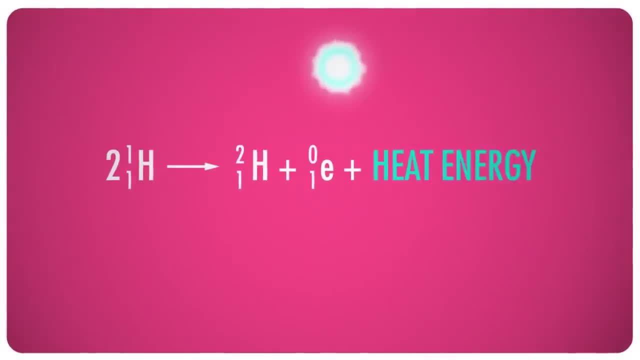 join to form an atom of deuterium, an isotope of hydrogen. This fusion of particles releases a positron and some heat energy in the process. Then another atom of hydrogen is joined to the deuterium to form helium-3.. 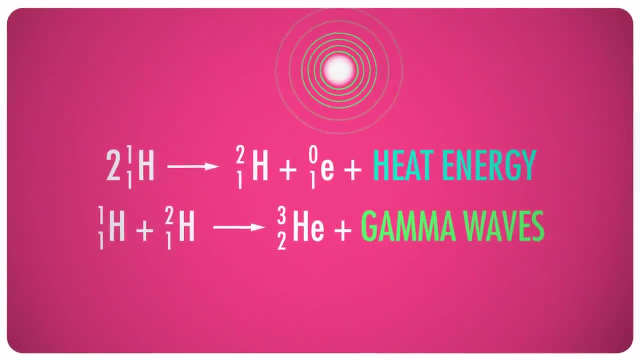 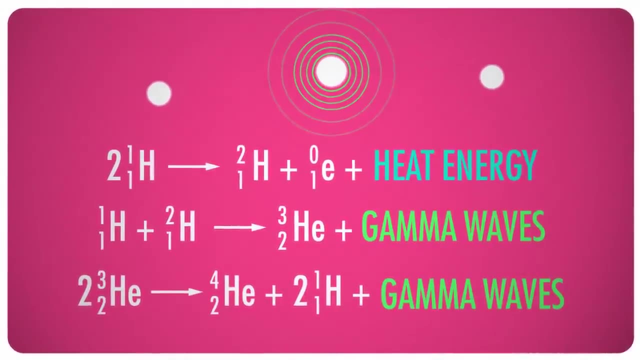 This step also releases a lot of energy in the form of gamma radiation. When two atoms of helium-3 are available, they join together to form an atom of helium-4, as well as two atoms of regular hydrogen, which then can be used to begin the process all over again. 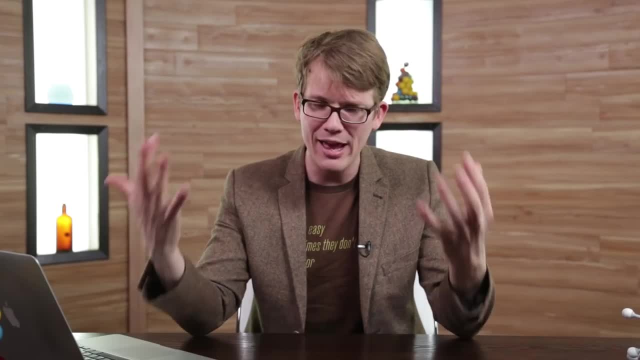 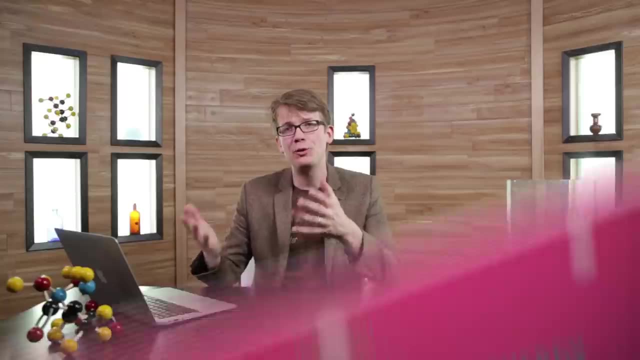 This final step also, as you might imagine, releases a large amount of energy in the form of mostly gamma radiation. So this is a chain reaction too, but it's not a self-perpetuating one. like we saw before, This reaction requires a total input of six atoms of hydrogen. 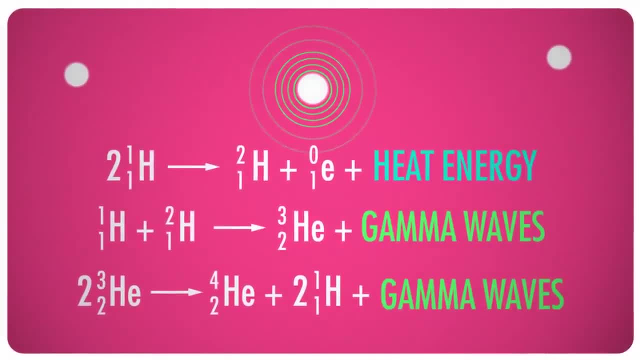 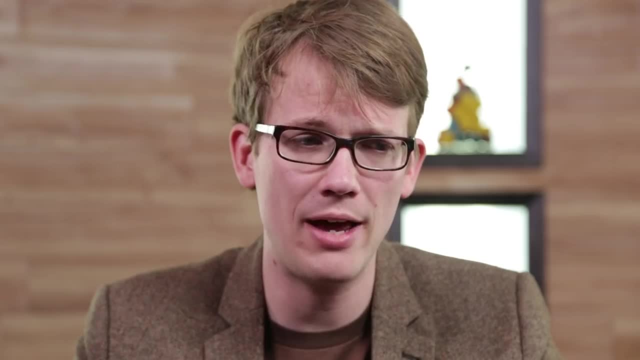 but it only produces two in the end, the remaining mass being released in the form of helium. For this reason, more fuel is always needed, which is why our Sun is going to run out of hydrogen In about five and a half billion years. We can produce fusion reactions here on Earth too, but they're not very useful for us because we haven't figured out how to control them. They're super useful if you just want to blow up a big city, though, Just to be clear, depending on your definition of use. One reason is, as you can see in the mass-energy graph, light nuclei that fuse together undergo a much larger energy change than heavy nuclei that break apart. That means their reactions release far more energy than fission reactions do, so much more that it's nearly impossible. 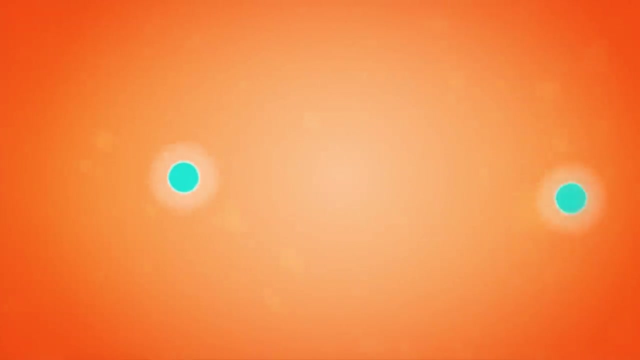 to contain and therefore use. Also, because fusion involves joining nuclei, the reaction has to overcome the really strong repulsion that naturally exists between their positive charges. For this reason, fusion reactions can only occur when particles collide at very high speeds or under very high pressures. 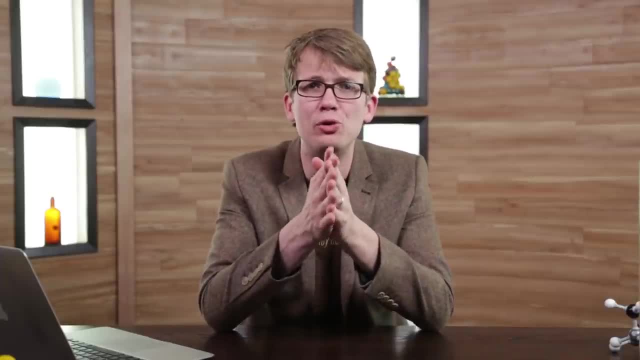 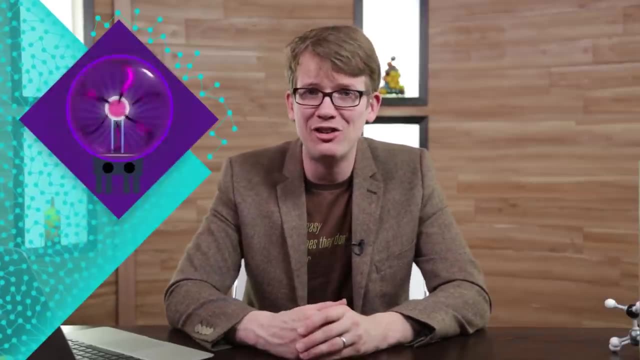 At these mind-blowing speeds the kinetic energy of the particles produces insane temperatures, like in the 100 million Kelvin range, at which point the material being accelerated actually exists in the form of plasma. So not only are those speeds really hard to reach, but material at that temperature. how do you control that? Which is why we can't use fusion for things like generating electricity, which would be super nice. We've only found applications for it when we don't need to control it at all, like in nuclear weapons. So, as you can tell, there is plenty of room. 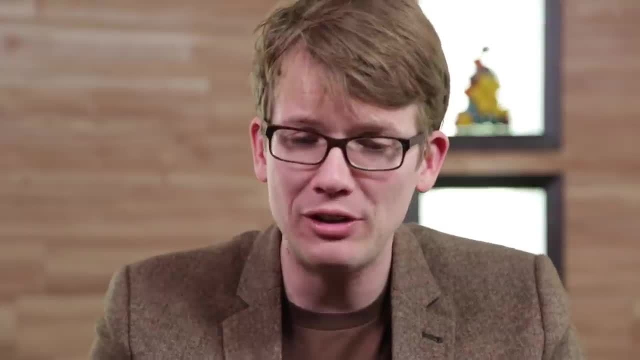 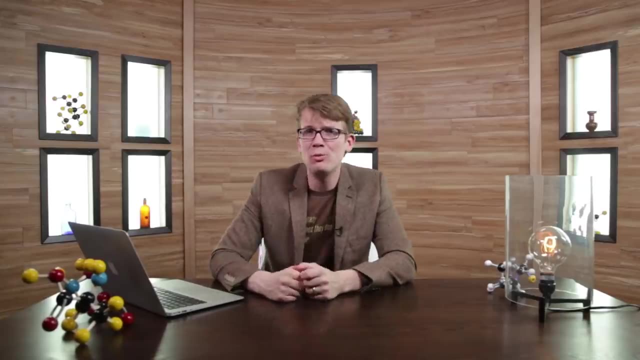 for new ideas in nuclear chemistry. Fusion would be really great because it would produce a lot of energy and you'd just get helium out of the process, and helium is awesome. How can we use radioactive materials more efficiently? Is there a way to achieve the speeds? 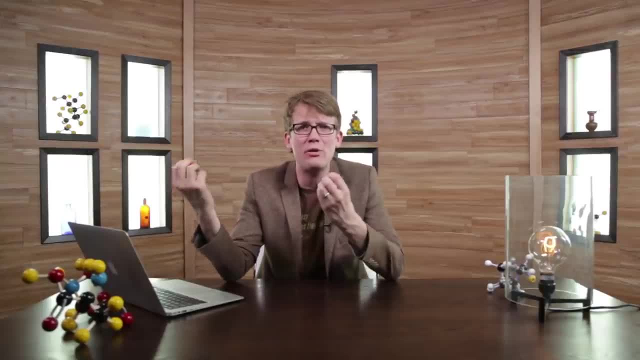 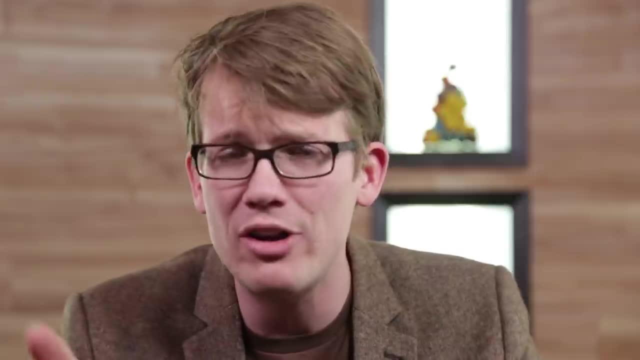 and manage temperatures that come with fusion, And how can we do this stuff without blowing our faces off? You've already taken the first step by learning the basics. It's up to you how far you want to go from here. Maybe you'll write the next: totally crazy. 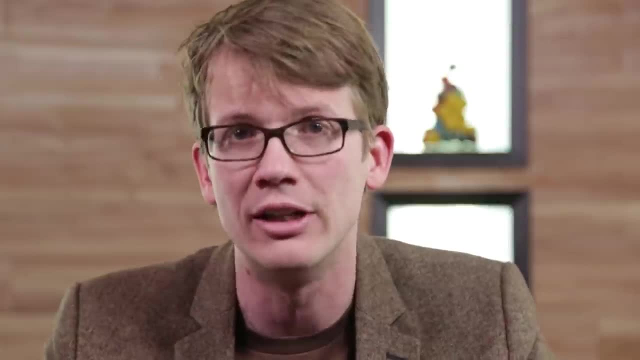 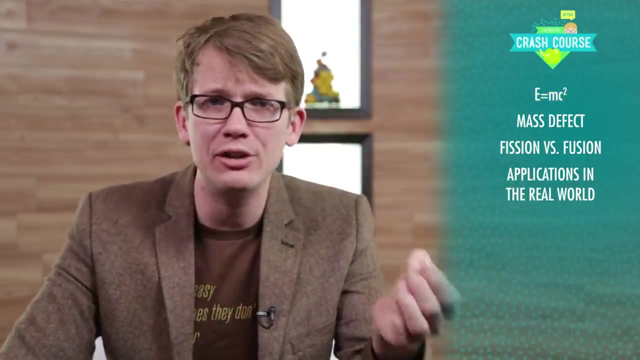 and genius and counterintuitive equation that takes us to the next level. For now, though, thank you for watching this episode of Crash Course Chemistry. If you paid attention, you learned how Einstein's famous formula helps us calculate the binding energy of a nucleus.